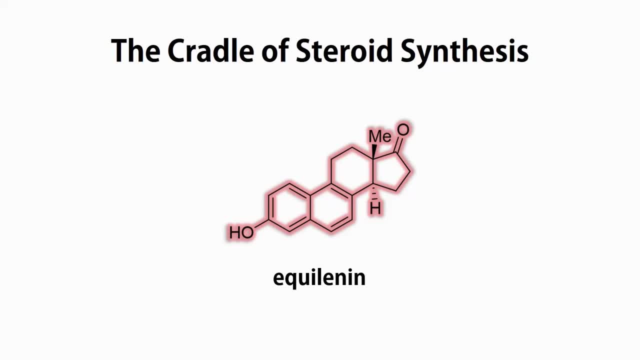 that exemplify more advanced concepts. These future videos will also include stereochemical and mechanistic discussions, which I know a lot of people requested. I'm leaving for a vacation soon, but I tried to squeeze in this video so it will be slightly shorter. 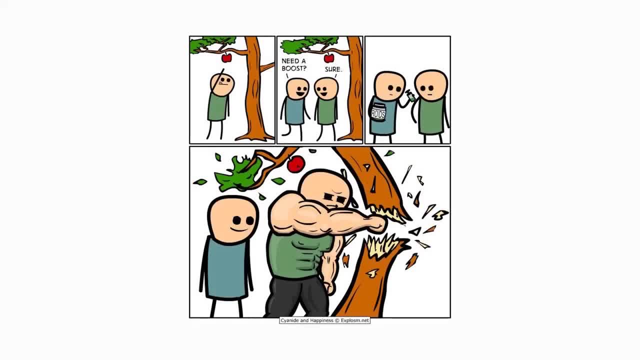 The accessibility of steroid hormones is not only important to the muscle head in your local gym, but has been paramount to the elucidation of a wide range of physiological processes in all kinds of animals. By the 1940s, steroids were one of the hottest targets amongst organic 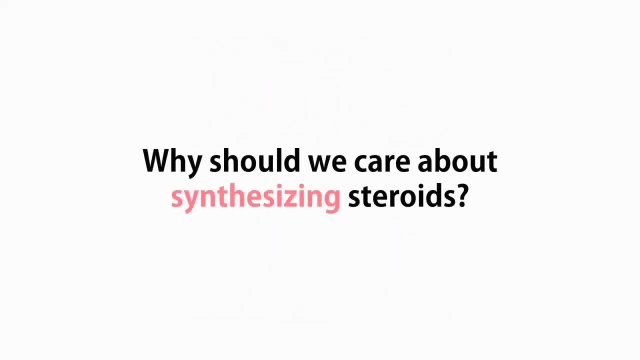 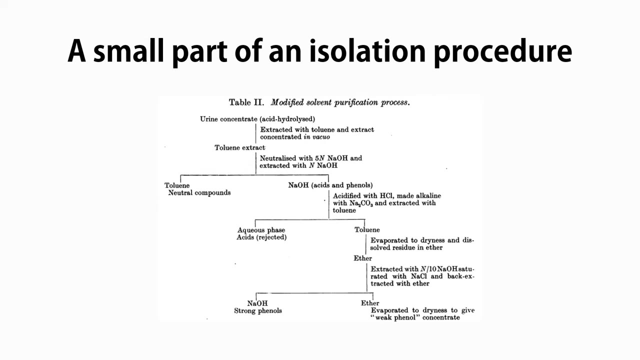 chemists. But why did people care about synthesizing steroids after all their natural products? right, Well, let's look at what situation we are in. Firstly, the actual procedure of isolating steroids from natural sources were tedious, to say the least. This involved a lot of extractions, concentrations, distillations, columns and 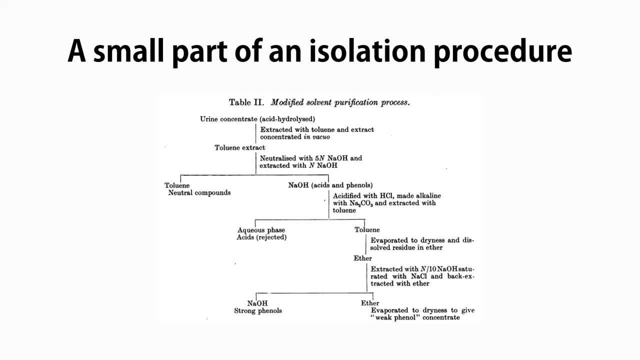 repeatedly playing around with pH values, Developing a procedure and analyzing your extracts and fractions consisted of injecting them into a castrated rooster to see whether this led to high growth-promoting effects on its red crest. I've personally visited an industrial, large-scale industrial facility in the United States and I've seen a lot. 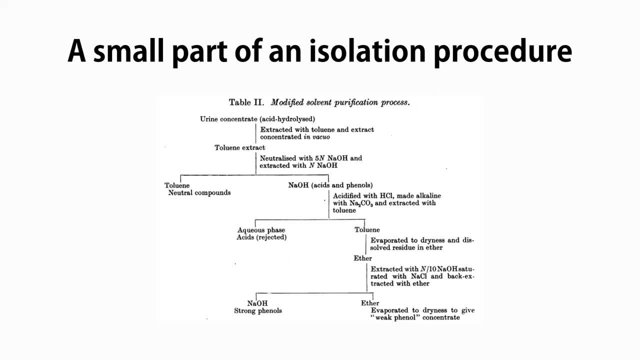 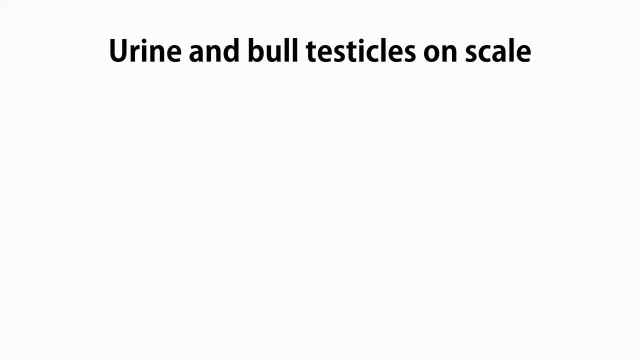 of people doing this. Let's say you're an industrial consultant and you're trying to follow a large-scale natural product isolation plan and, oh dear, is it a lengthy process. Let's say you were totally cool with isolating steroids from nature. Well, go ahead and take a look. 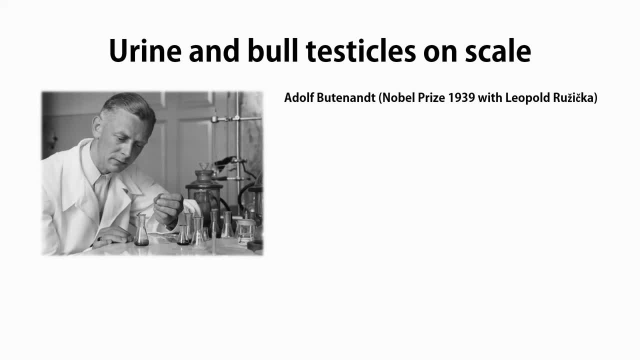 at the required scale and your very practical yields. The German biochemist and Nobel laureate, Adolf Butenand first isolated the steroid androsterone in 1931. To obtain 15 mcs of crystalline material, he had to process 25,000 liters of urine. To obtain 15 mcs of crystalline material, he had to process 25,000 liters of urine. The first step was to isolate the steroid from nature. But this was not the only way of isolating steroids. The first step was to isolate the steroid from nature To obtain 15 mcs of crystalline. 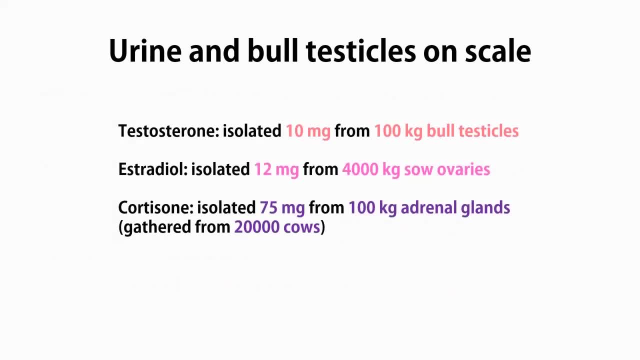 Similarly ridiculous amounts of materials were required for other steroids as well. To put these numbers into perspective, the isolation of 75 mg of cortisone required adrenal glands from 20,000 cows. Because we're already talking about insane natural product isolations, I want to quickly. 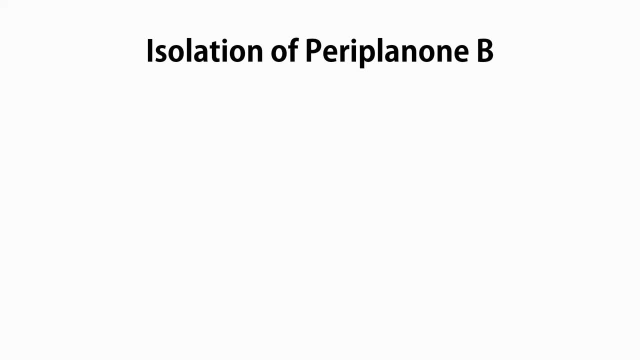 mention my favorite one, the cockroach pheromone periplanon B. After 7 years of work, 200 micrograms were isolated from 75,000 female virgin cockroaches. It's a really potent pheromone, though, as femtogram quantities are sufficient to send male cockroaches. 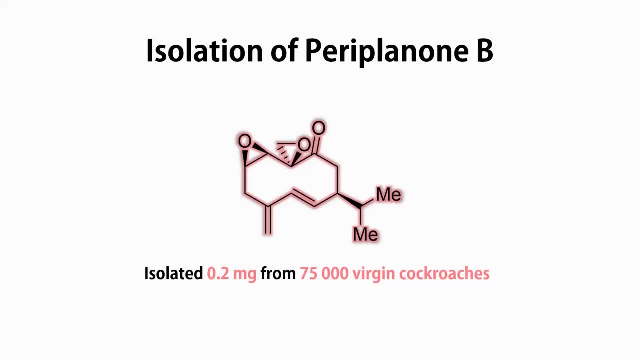 into a sexual frenzy. The total synthesis of periplanon B by Clark Still in 1979 is a classic that some of you probably have heard about already. So now that we've established that, unless you want to take out a whole farm or collect, 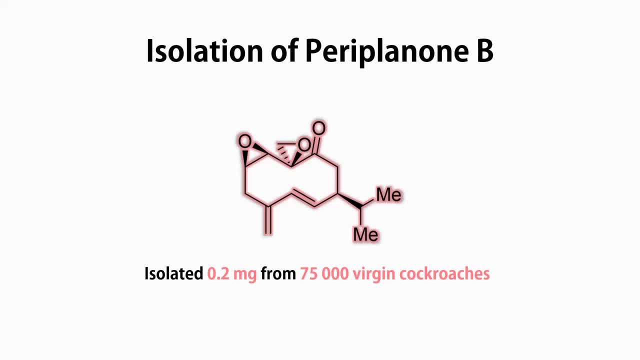 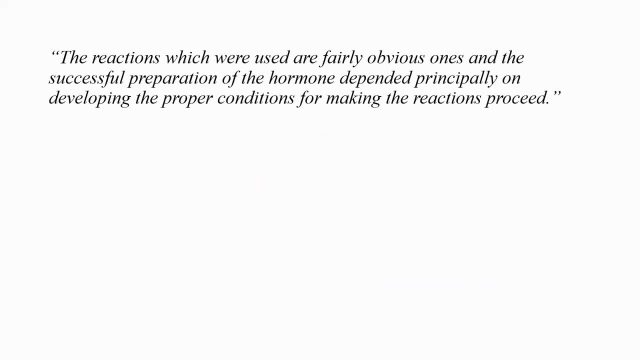 a small country's worth of urine. to get your hands on some steroids, we need to make them synthetically. Before we dive into this video's synthesis, let me give you some more context. first, This synthesis for some people constitutes the end of the pre-WWII era in organic chemistry. 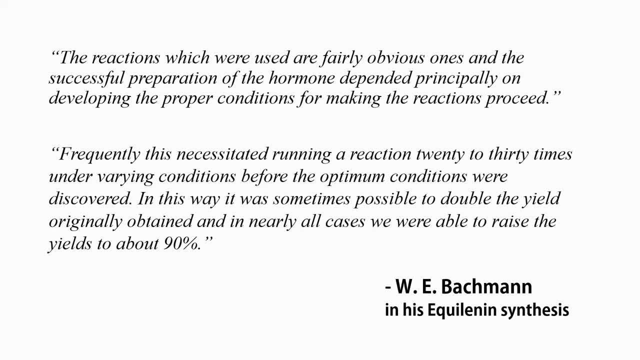 Up to this point, total syntheses were closely tied to structural proof, so chemists employed robust reactions without very creative design. This notion soon changed after the Second World War. The isolation of more complex natural products and insights into mechanistic organic chemistry catalyzed the development of novel reactions and strategies. 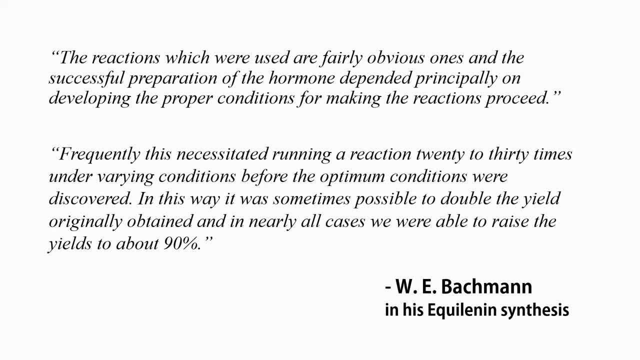 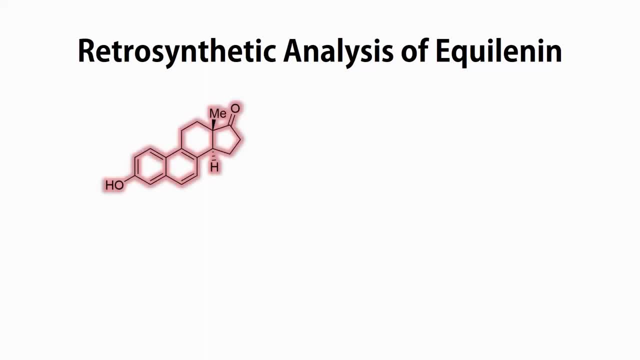 In turn, it was possible to plan longer and more sophisticated sequences. Let's take a look at the first total synthesis of a steroid and one of the most complex natural product syntheses at that point: the Bachmann synthesis of equilenin from 1939. 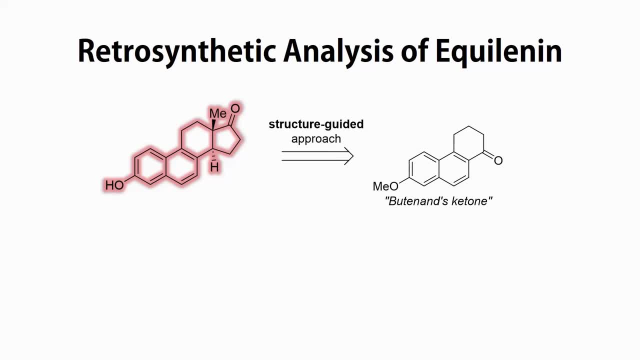 Bachmann employed a structure-guided retrosynthetic strategy By choosing this known ketone as a starting material. basically, all he had to do was to introduce a methyl group. This was the first ketone to be used as a starting material. The second ketone to be used was to fuse one additional ring to complete the steroid. 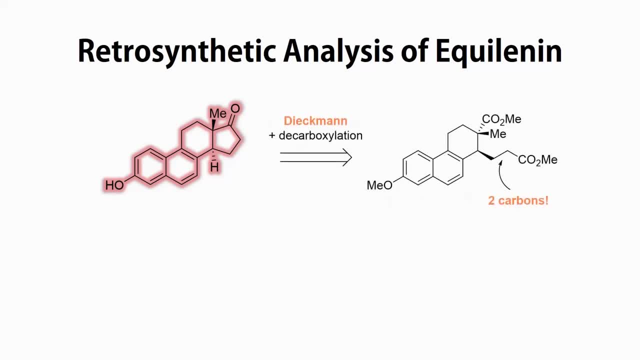 nucleus. To this end, he envisioned a Diekmann cyclization and decarboxylation process starting from this diester. To connect this intermediate to the known ketone, two carbon homologations had to be incorporated. One of them was accomplished by employing the recently discovered Arendt-Eichstatt homologation. 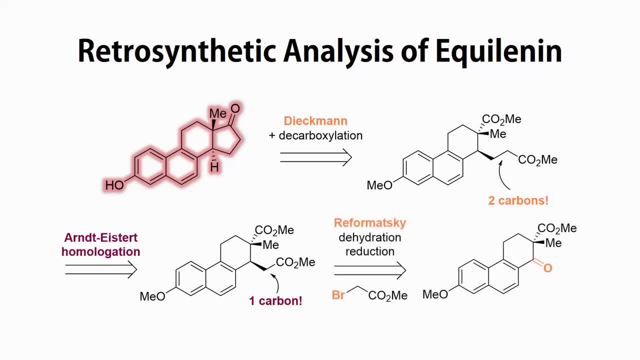 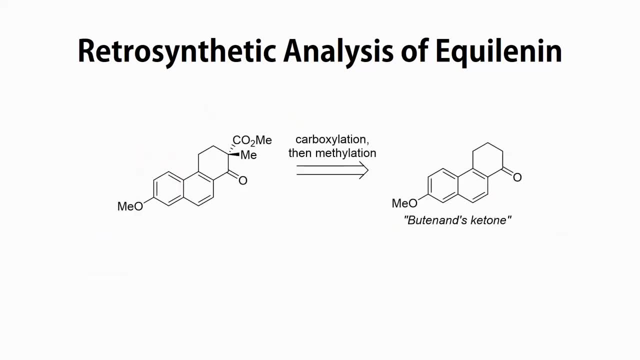 The other homologation consisted of a Reformatsky reaction dehydration reduction sequence. The use of this beta-keto-acid as an intermediate allowed for facile construction of the quaternary center via enolate chemistry. Let's take a look at the forward synthesis and how the so-called Putanon's ketone can. 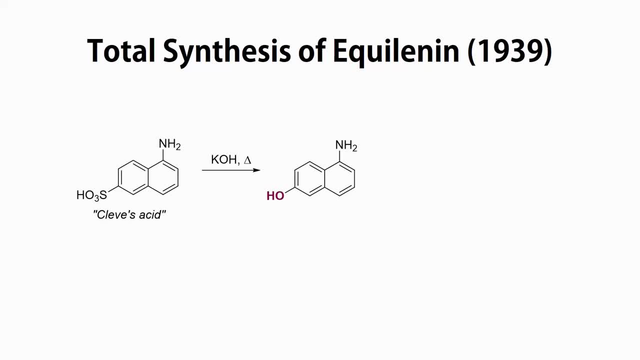 be accessed. The preparation commenced with hydrolysis of this naphthylamine sulfonic acid, called Cleaves acid, Subsequent acetylation of the amine, methylation of the naphthol and deacetylation of the amine. 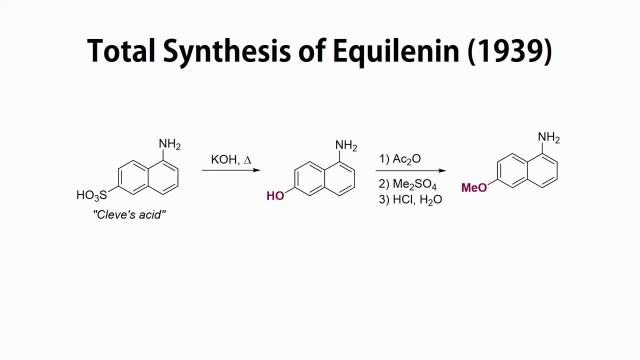 gave the immunoprotected amine. There will be another cool play around with protecting groups. I hope you enjoyed this video. Nucleophilic substitution of the corresponding diazo species in a Sandmeyer reaction. give this aryl iodide. 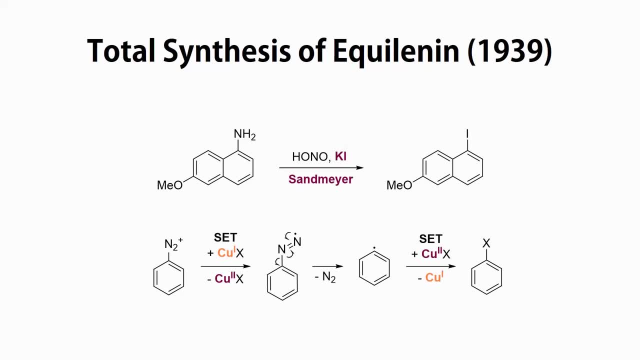 The Sandmeyer reaction is quite interesting. With chloride bromide or cyanide nucleophiles it requires copper I catalysis and proceeds with a radical mechanism. Employing iodide as a nucleophile doesn't require copper catalysis and is quasi-autocatalysed. 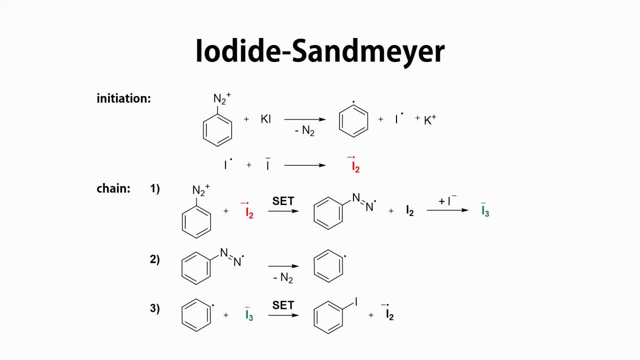 The mechanism is a bit more complicated, but that's the reason why we're using potassium iodide and not a copper source. There are modern variants of this reaction that enable, for example, the trifluoromethylation of arenes, so it's quite useful. 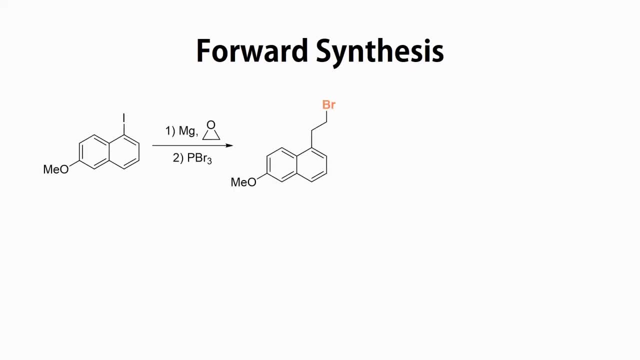 The aryl iodide Grignard reagent was reacted with ethylene oxide and the resulting alcohol converted to the bromide. Substitution with diethylmalonate, decarboxylation and chlorination give the acyl chloride which was subjected to a Friedel-Crafts acylation. Similar to the Woodward synthesis of lysergic acid. we've talked about the deacetylchloride, which was subjected to a Friedel-Crafts acylation Similar to the Woodward synthesis of lysergic acid. we've talked about the deacetylchloride. 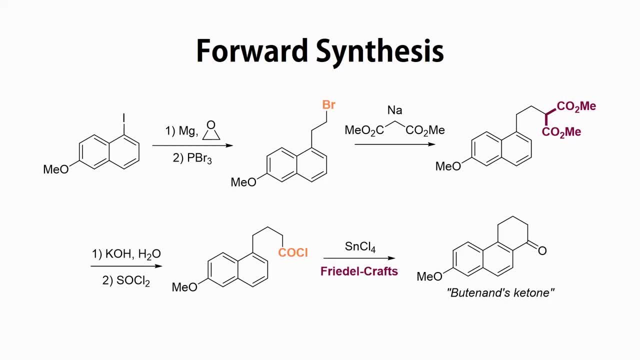 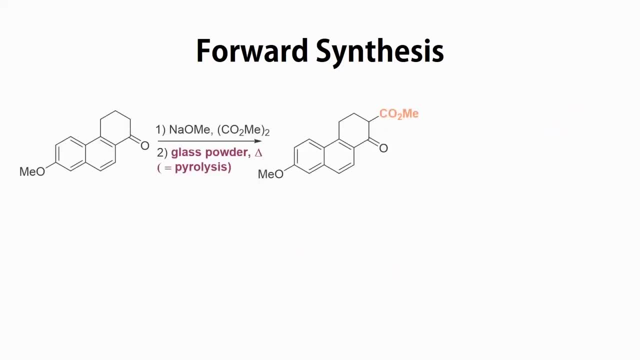 and this time tin tetrachloride is the Lewis acid of choice. So now that we've arrived at our ketone starting material, let's start the actual synthesis of eqalenine. The ketone was converted to the β-ketoacid via a reaction with methyl oxalate and pyrolysis. 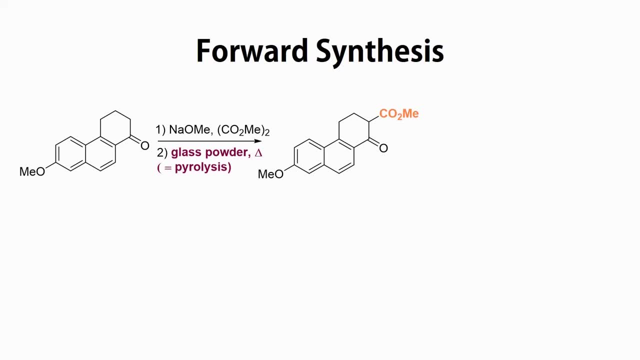 to eliminate carbon monoxide. Nowadays one would just use an activated form of methyl carbonate. A simple methylation installed a collider nary center, reformatsky reaction. elimination, ester hydrolysis and reduction with sodium amalgam resulted in the first homologation. 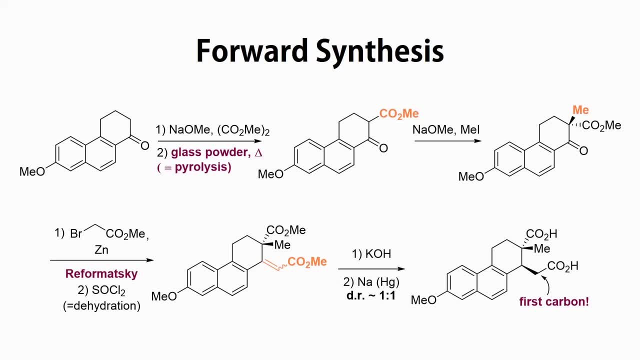 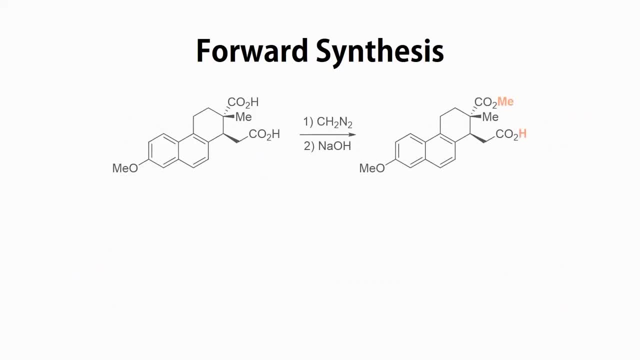 The DR of this reduction was about 1 to 1, so diastereoselectivity in this synthesis was not a problem, but not really thoroughly planned either. Now, remethylation of both free acids and selective hydrolysis of the less hindered ester.